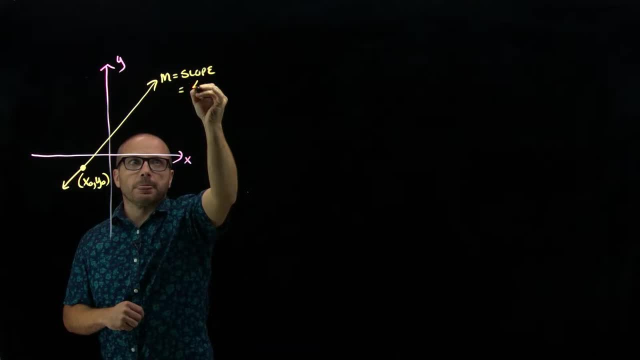 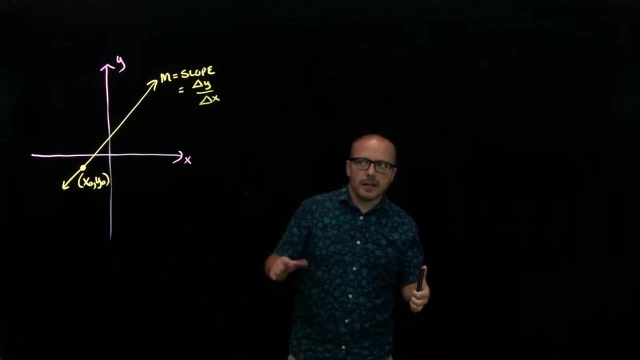 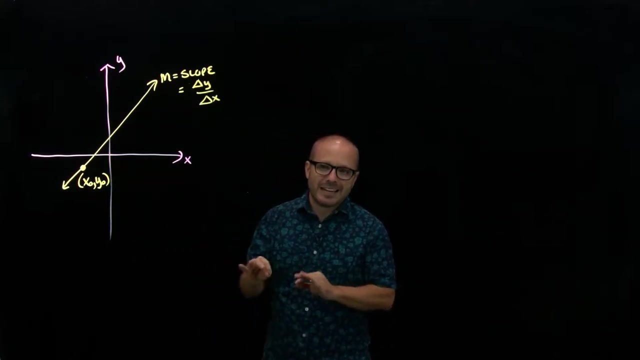 some change in y over, change in x, right, Rise over, run. Those two things define a line. If you have, if you know the tilt and where it's located, you have a line. and actually vertical lines don't even have a slope right. So let's think about this: What would be true of any other? 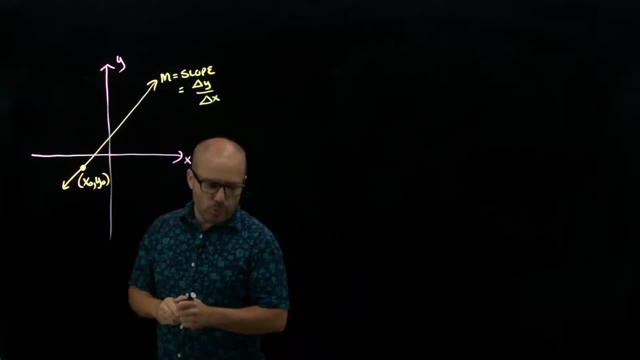 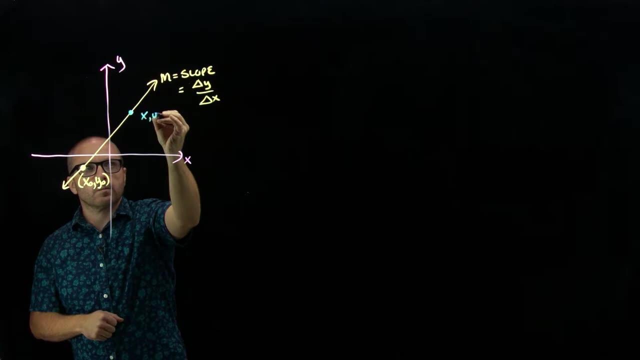 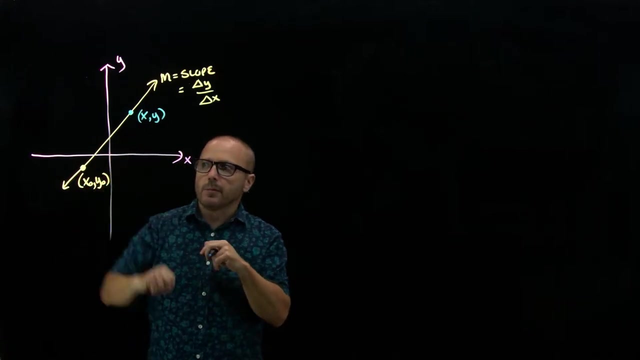 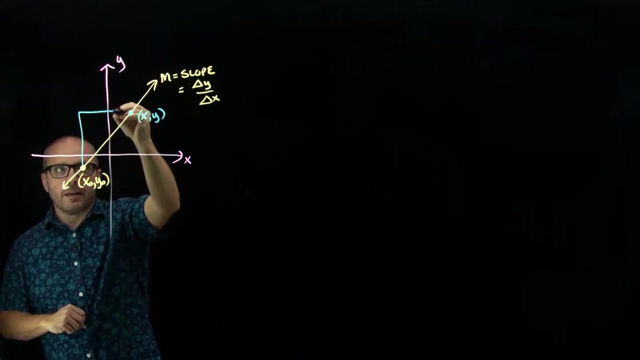 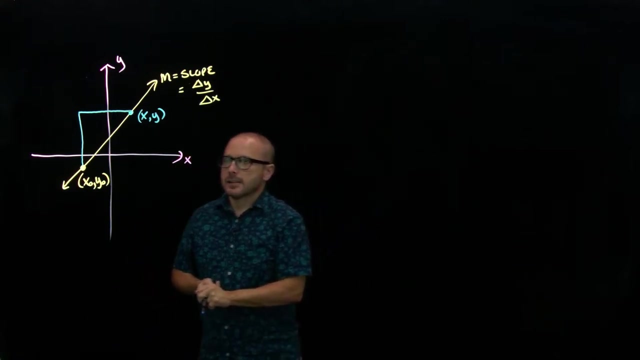 point on that line. So any arbitrary point I can draw, call it x, y To get from the point that I know to any other point. there would be some amount of up and down and some amount of left and right. right Now, what's going to be true? 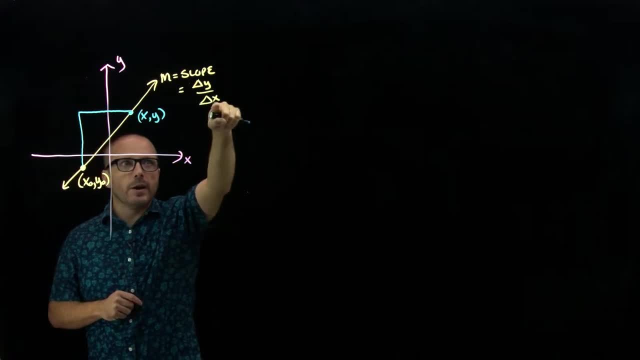 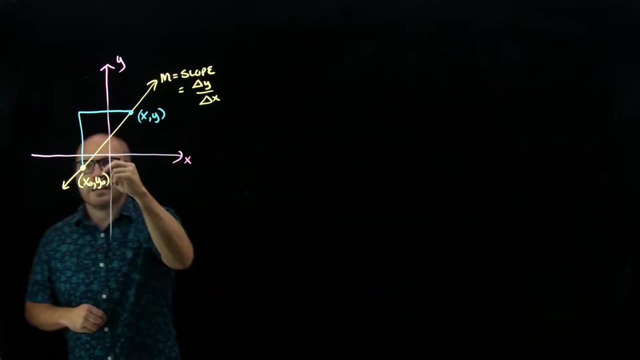 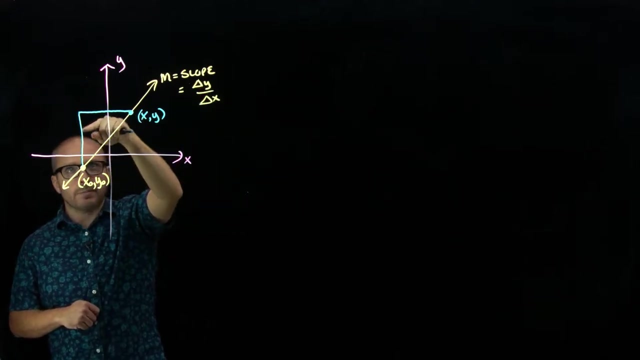 true about these two quantities? Well, their ratio should be delta y over delta x. So what that tells me is that it may not be exactly delta y over delta x. excuse me, each of these may not be exactly that delta y or that delta x, but their ratio is always the same, right. 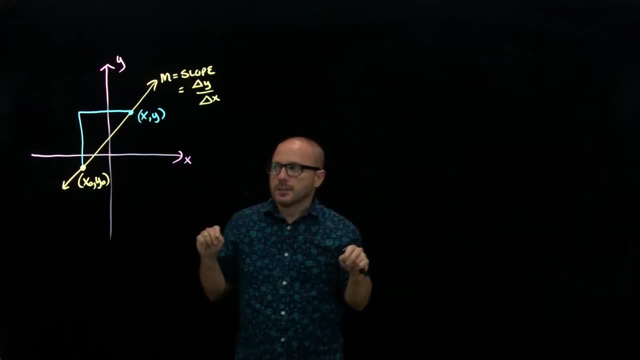 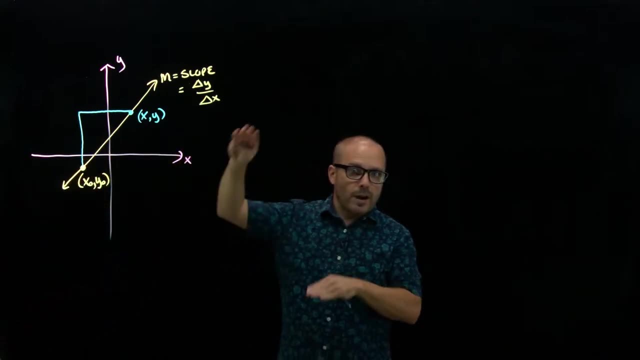 That's the point of a line. The slope is constant. So no matter where I'm at, if I go to that point or that point or that point or this point or a point way down here, the ratio of the change in x and change in y will be the same as whatever this fraction is. That's what it means to be a. 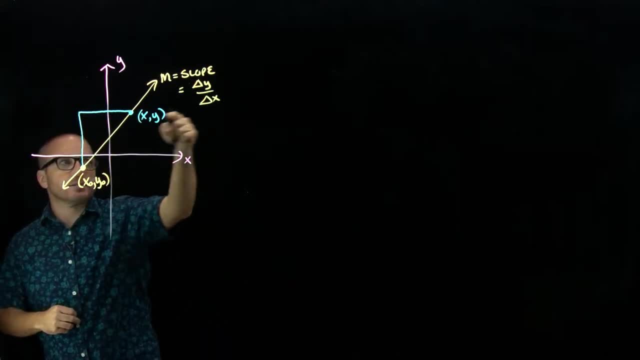 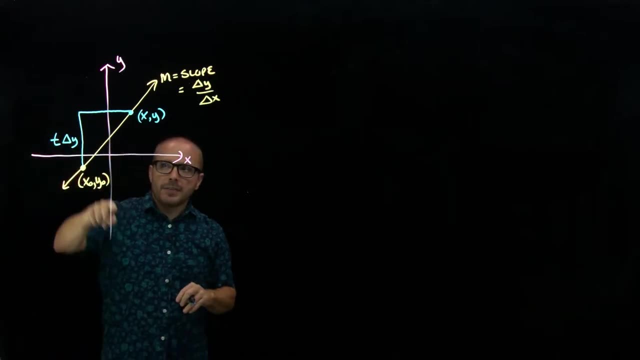 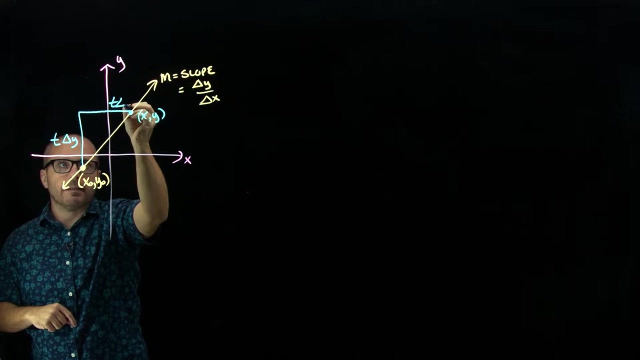 line. So that means that this up and down has to be some multiple of this- I'll say t times delta y, And this left right has to be some multiple of that delta x. So I'm going to call it t delta x, That quantity. 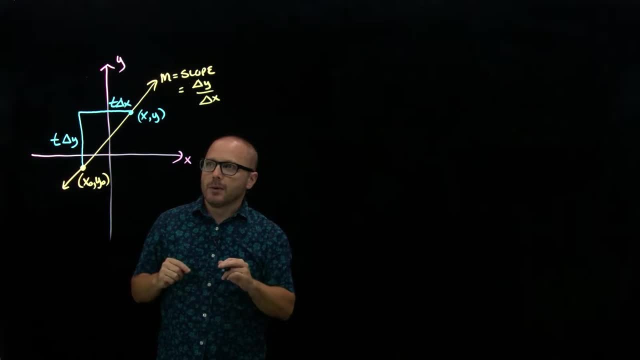 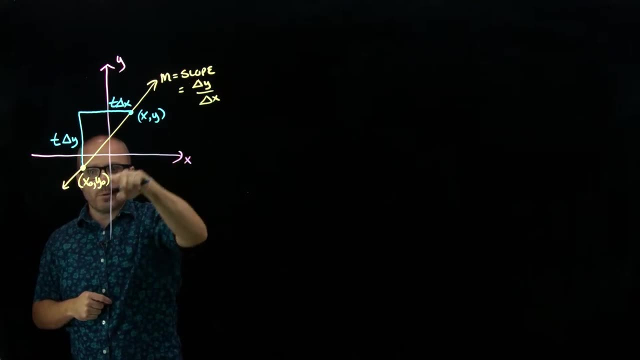 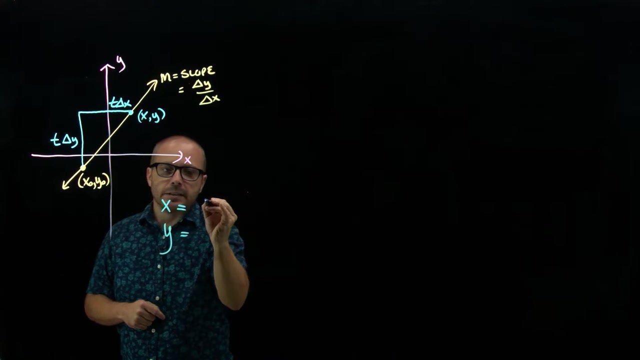 And that quantity. So what does that mean? Any other point is to go from any arbitrary point to my known point. I am just adding some multiple of delta x to the x and some multiple of delta y to the y. So that means what's true of every point on the line is: it's our, excuse me, our initial. 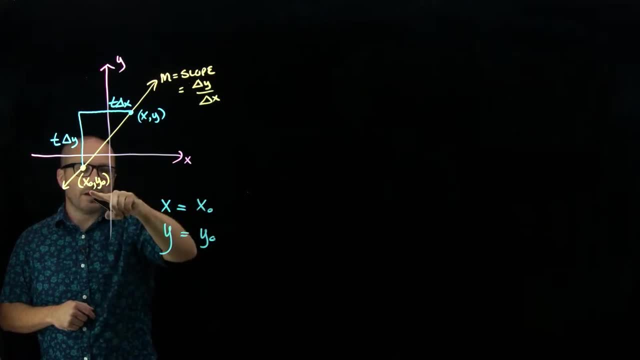 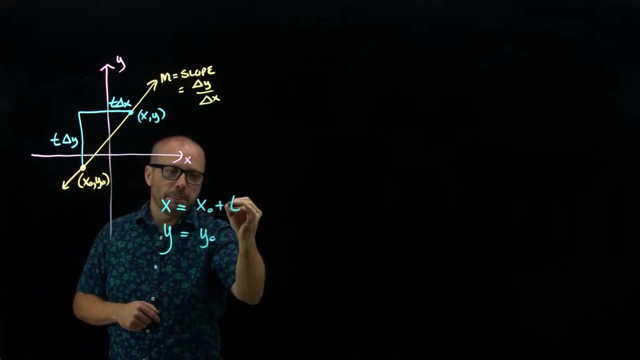 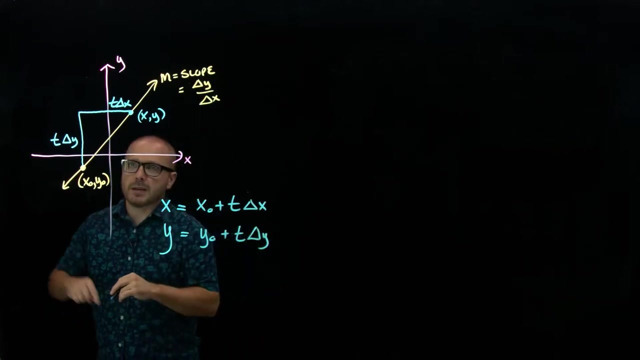 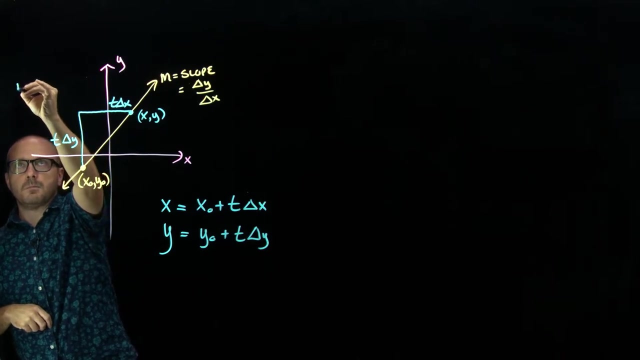 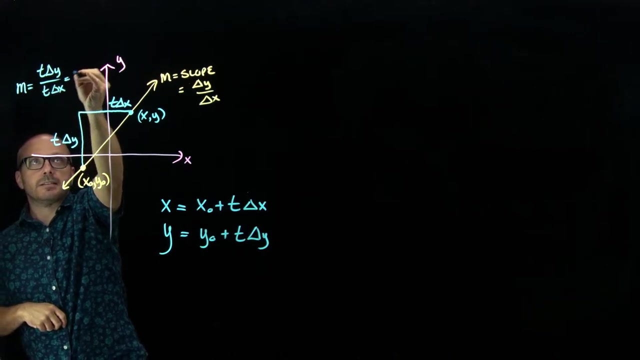 point. right, Like I just said, that backwards, but either way, But from our initial point, from our known point, I would add some multiple of delta x and add some multiple of delta y. right, Because even if these aren't exactly those numbers, the ratio right- t delta y over t delta x- is 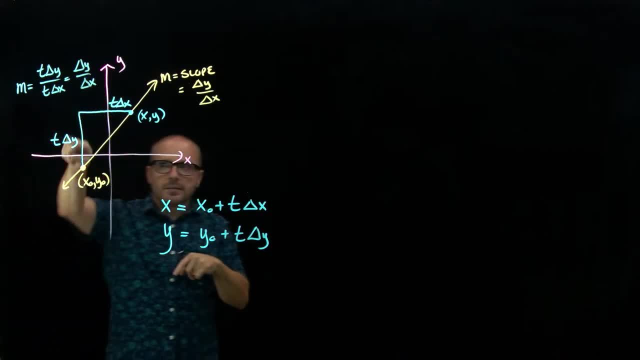 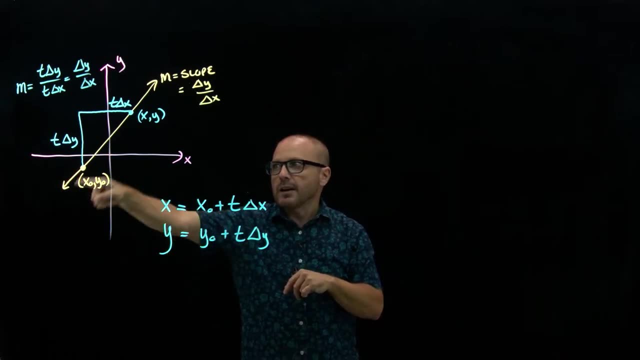 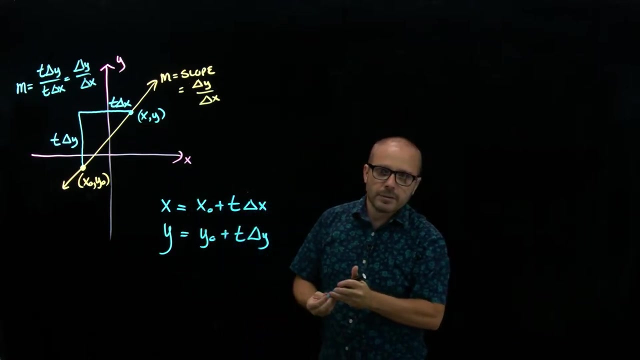 delta y over delta x, So that's maintaining that slope everywhere. So in order for that to be true, every x- y pair that we can generate on that line should be our original point, plus some change in x and y that are a multiple of the quantities in this fraction. 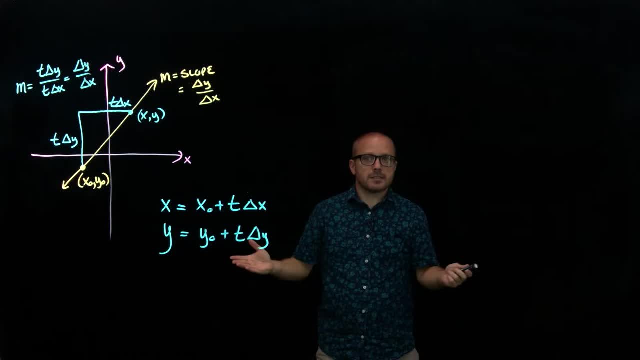 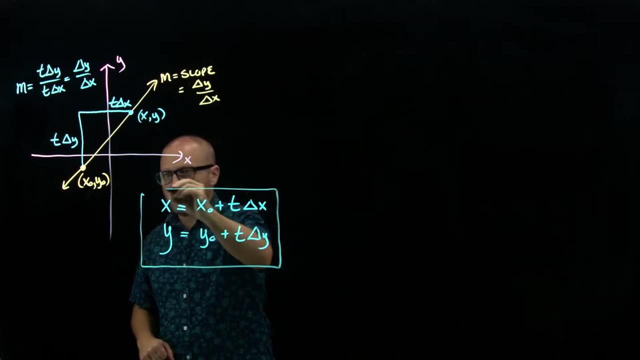 defining our slope, And it's as simple as that. There's our equation of the line And actually, if you want to go into 3D- which we won't in here, but you would just have a third equation- z equals z, naught plus some, 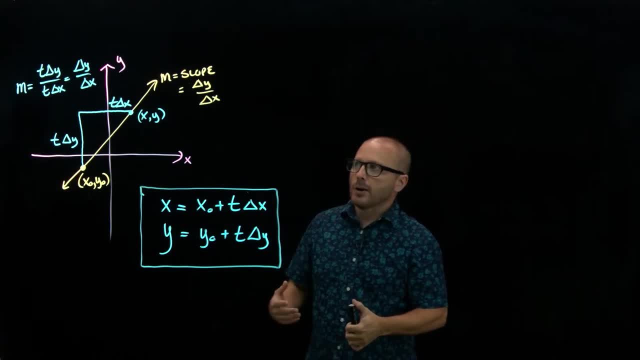 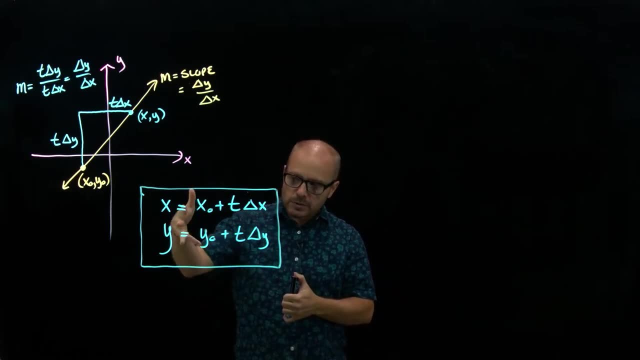 multiple of the change in z. Now slope goes out the window. in 3D We're going to use vectors to describe the orientation of a line, but it's still the same concept of you. start at some x, y, z and. 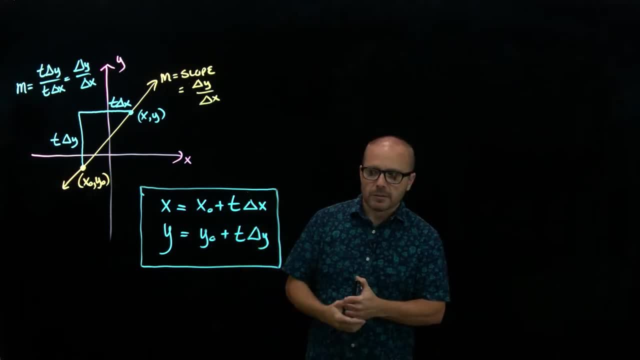 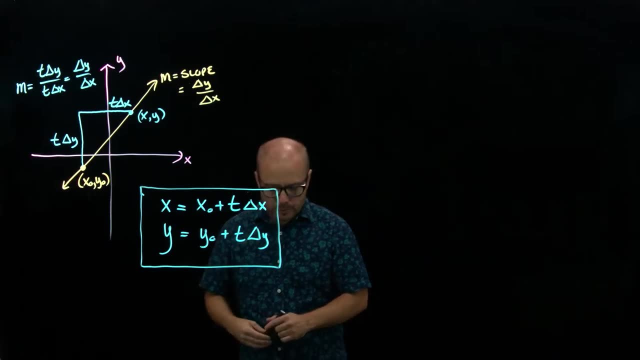 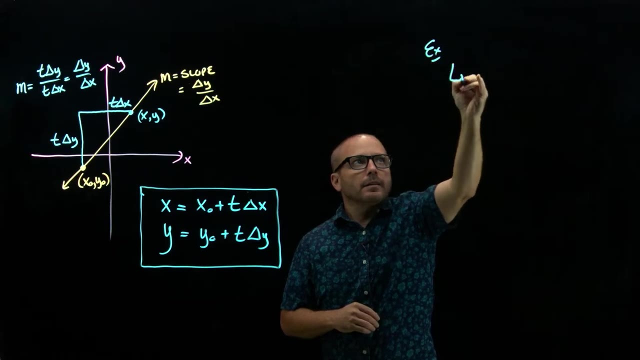 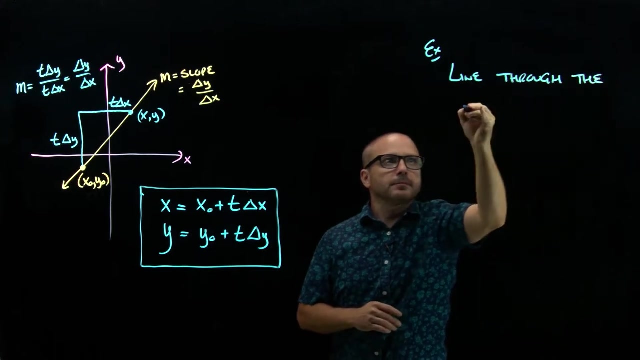 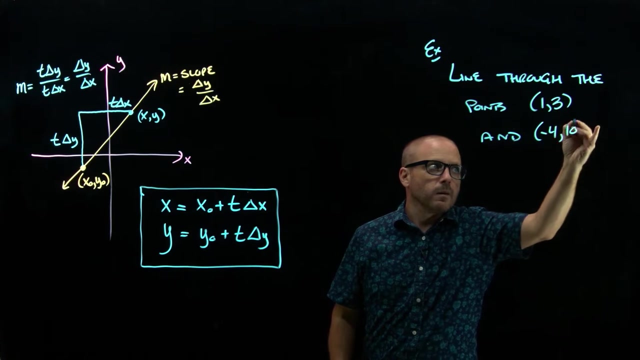 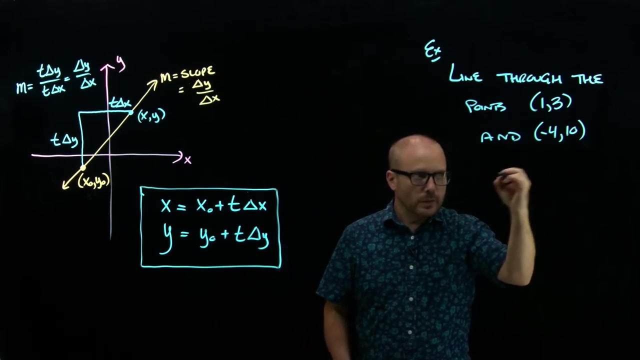 you move some constant amount along all three directions. Not the same amount, but constant, Okay. so let's look at an example. Let's find the line through the points 1, 3 and negative 4, 10.. So let's draw a picture. We don't really need to From the formula, we can just write it, but I just want. 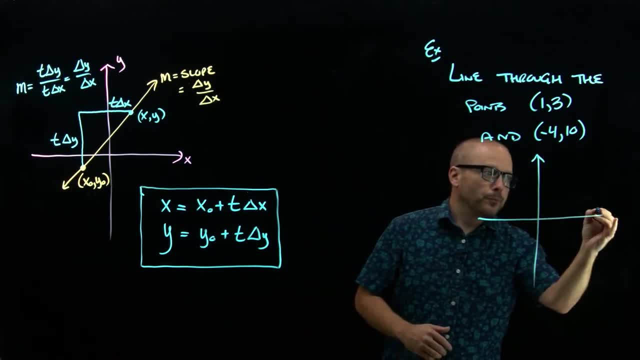 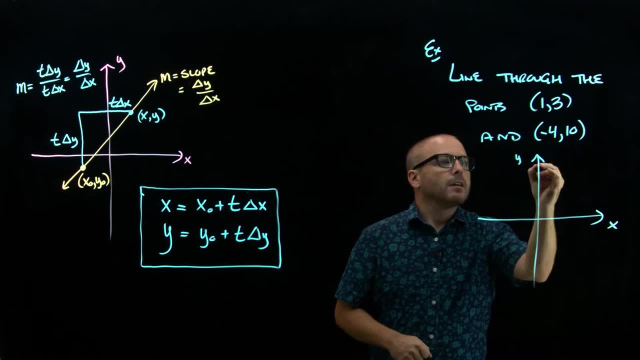 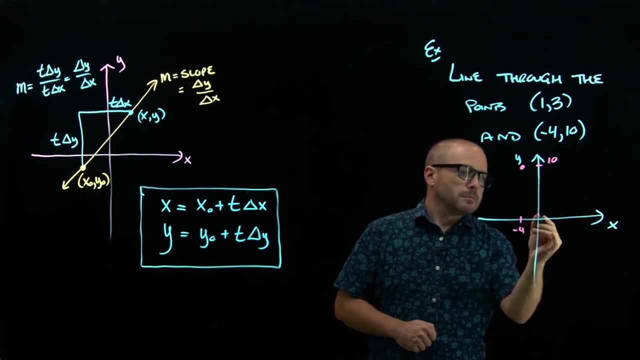 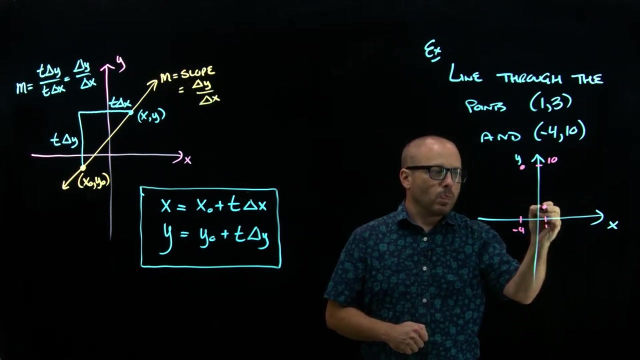 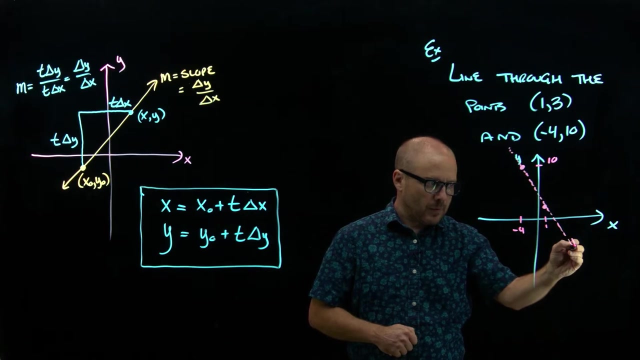 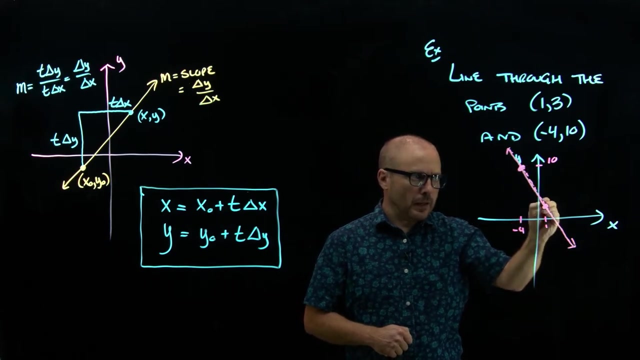 to think about what we're doing here. So negative 4, 10. Right there And 1, 3. About there. We're talking about this line From there to there, And I haven't really mentioned anything about direction of motion. Right now we're. 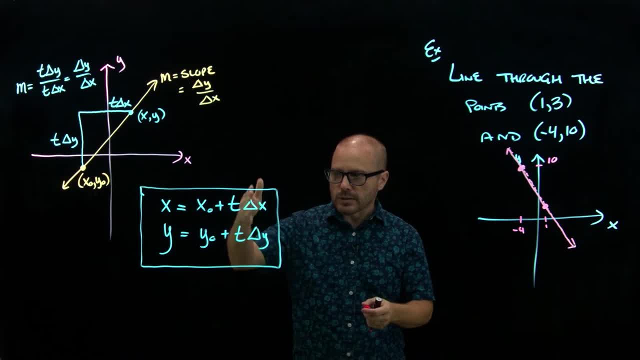 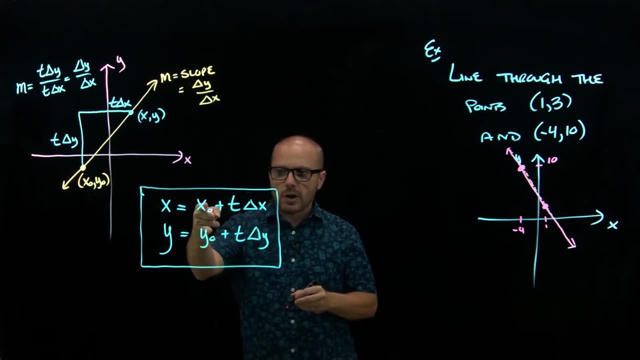 just going to be interested in getting the line. Depending on how you set this up, you could easily make this go one way or the other. So what would be our equation? Well, we need the starting point. Well, we have two points, so take your pick, whichever one you want to use. 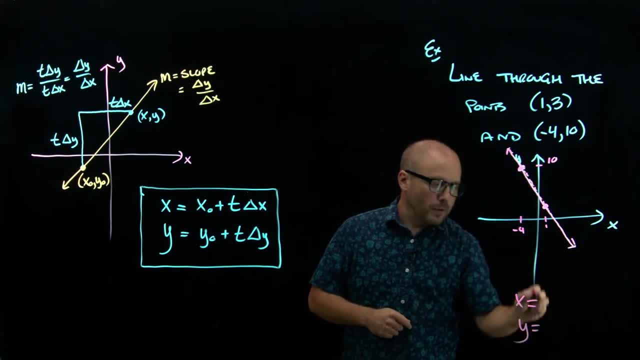 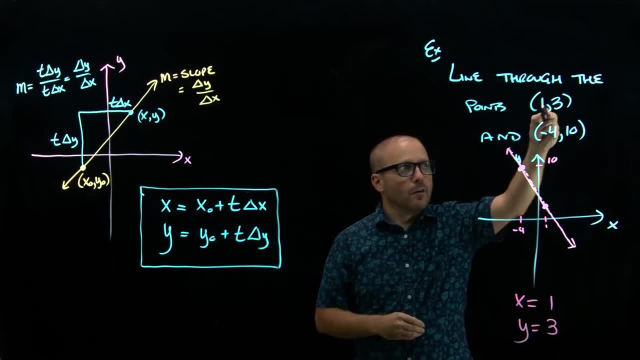 So let's say I want to start with the point 1, 3, for example. Now what is my change in x and change in y as I go from point 1, 3 to point negative 4, 10?? 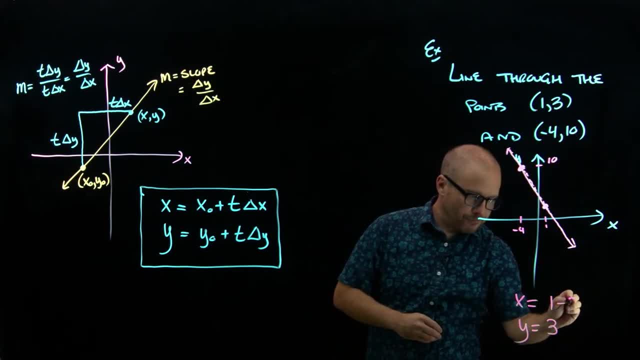 Well, to go from 1 to negative 4,, you subtract, 5. Subtract, 4. Subtract, 5. Subtract, 5. Subtract, 5. an X. and to go from 3 to 10, you add 7.. As simple as that. we have the parameterization. 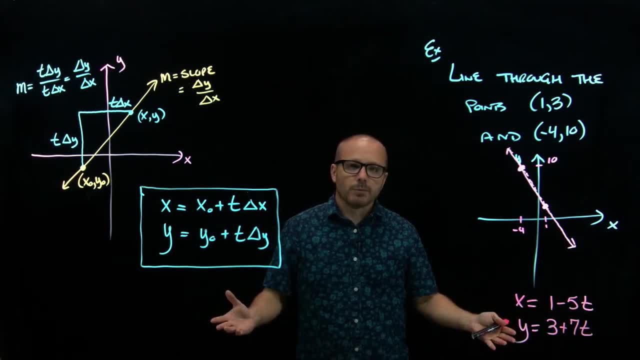 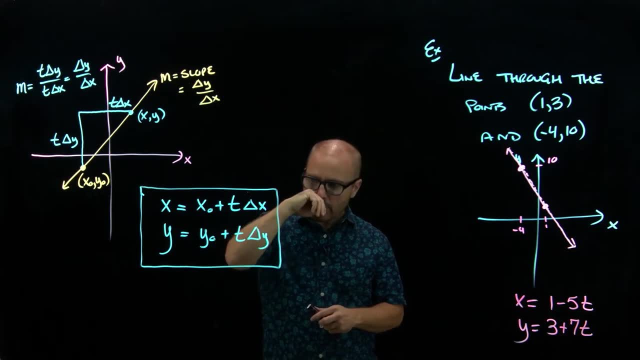 of our line. Now, there's many ways you could have parameterized it because, remember, this could be any point and really all that has to be true is the ratio of Delta X and Delta Y. Delta Y over Delta X should be your slope, So 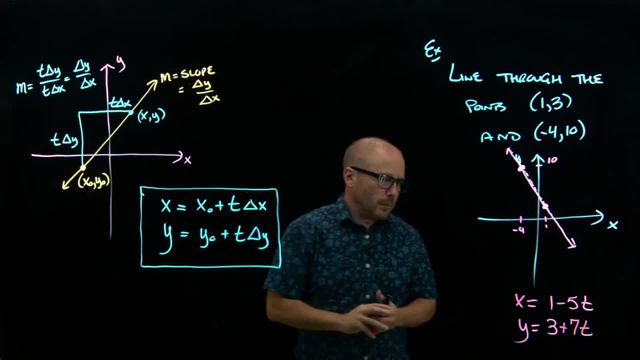 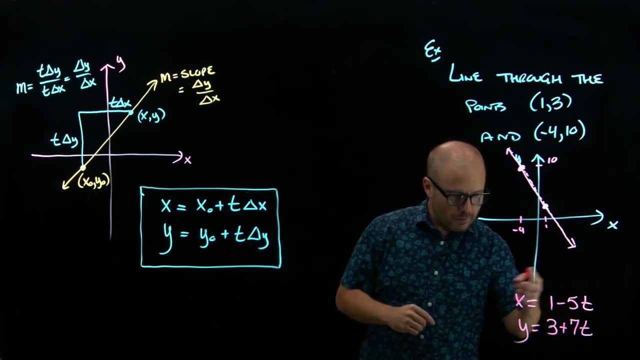 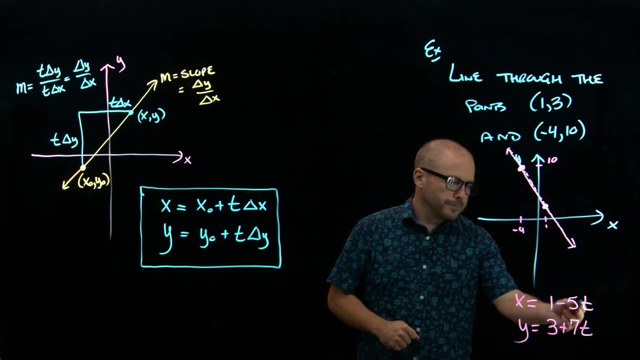 really any constant multiple of that works as well. That would just speed up or slow down your your parameterization. Now, one important thing about the method I just used here is: what will always be true is at time 0, when t is 0, you're at. 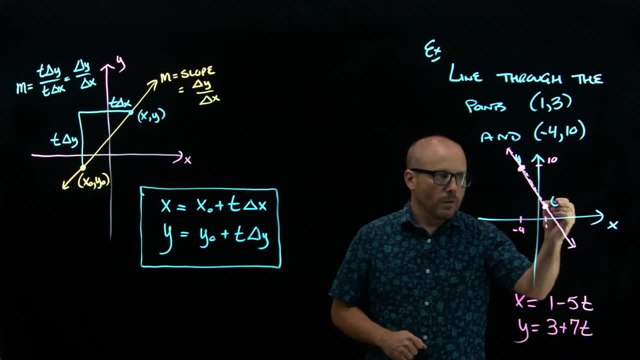 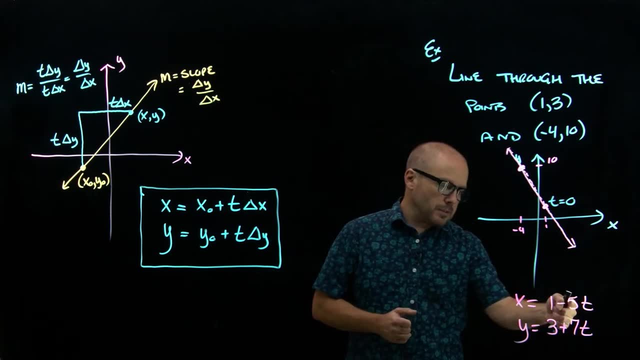 the point 1, 3.. So you're there at time 0.. The point that you pick is actually your location at time 0 and, because I make this the change, that you need to move to the other point, that's where you are when t is 1, right, 1 minus 5 is negative. 4, 3 plus 7 is 10.. So you're.